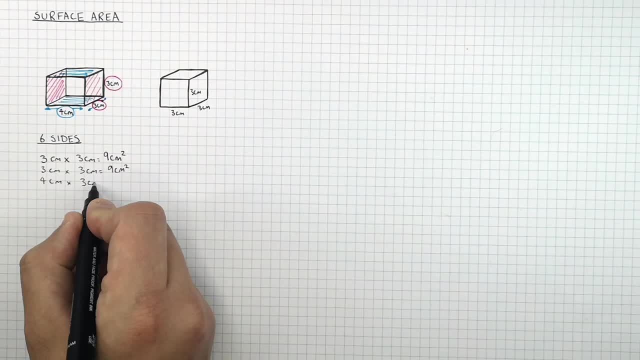 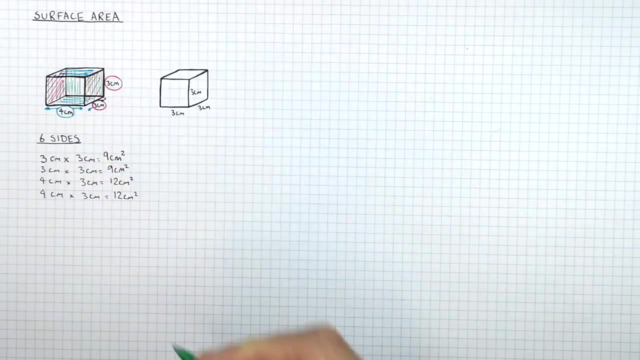 So you do four centimetres times three centimetres. So that's four centimetres the length times three centimetres the width, which gives you a surface area of each of those faces of 12 centimetres squared. So to work out the surface areas of the remaining two faces, 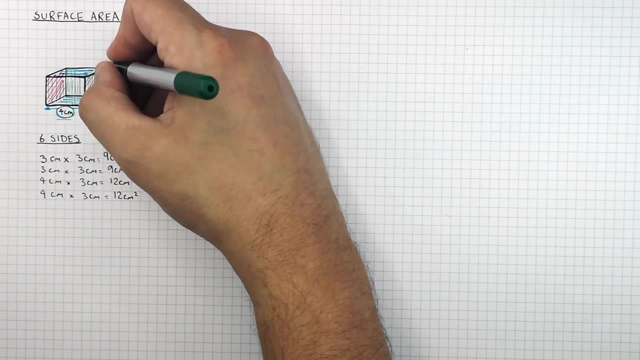 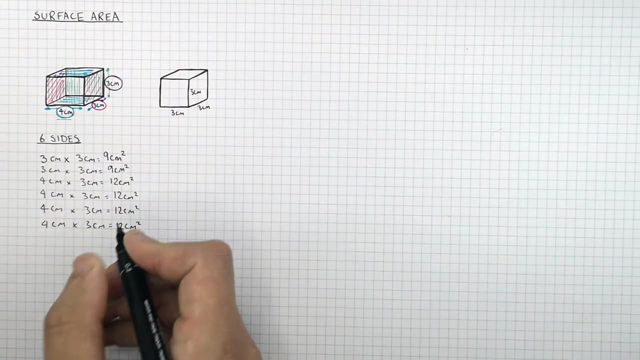 You do 4 centimetres times by the height, which is 3 centimetres, That will give you an area of 12 centimetres squared for both of those faces. So to work out the total surface area for this cuboid, you add all the surface areas of the faces together. 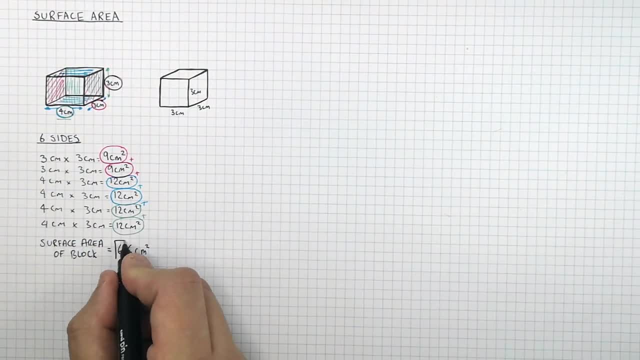 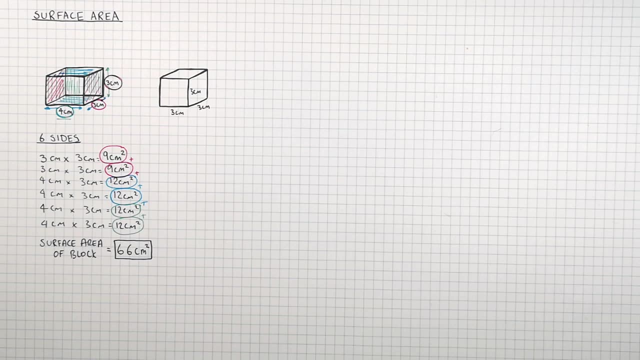 So the surface area of this block is 66 centimetres squared. Pause the video to calculate the surface area of this cube. The answer will follow, Because this is a cube of 6 sides measuring 3 centimetres by 3 centimetres by 3 centimetres. 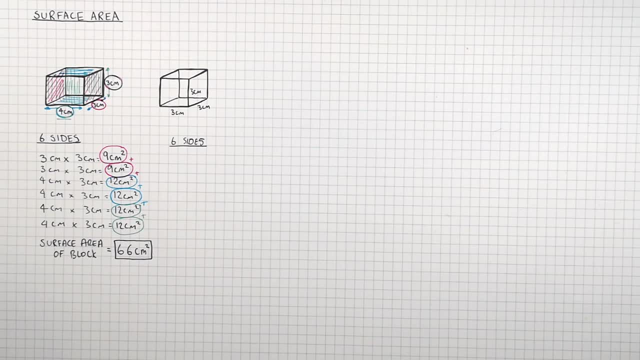 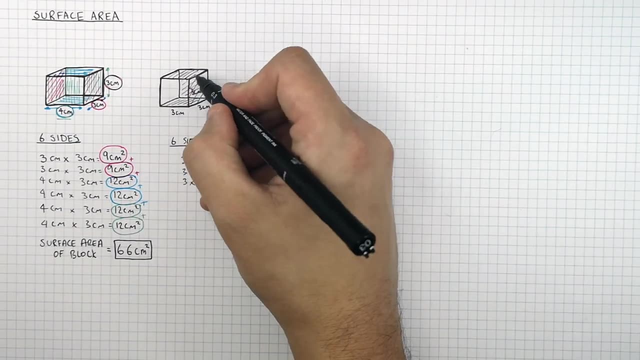 you only need to work out the surface area of one face and then multiply that by 6.. So 3 times 3 is 9 centimetres squared, which means that every face, as you can see here, is going to have a surface area of 9 centimetres squared. 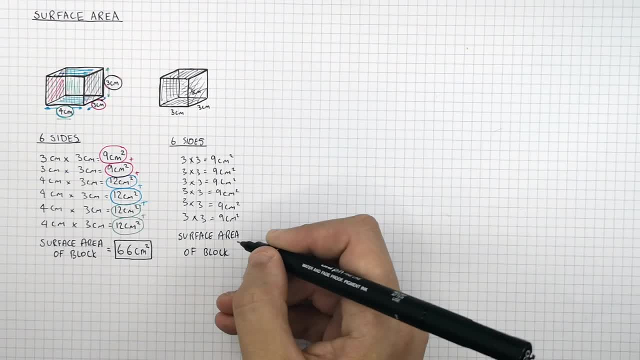 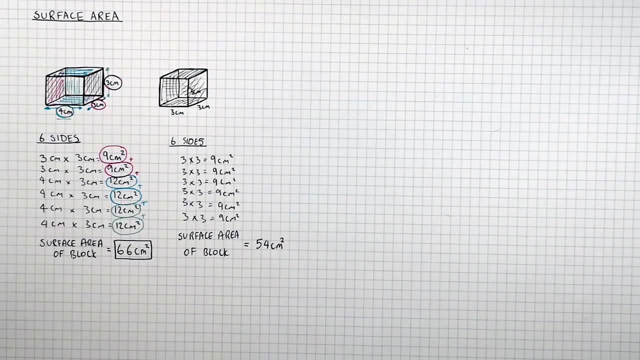 So to calculate the surface area of this block, you simply do 9 centimetres squared times by 6. So that gives you a total surface area of this cube of 54 centimetres squared. It's question time. Tempt these questions to check your understanding. 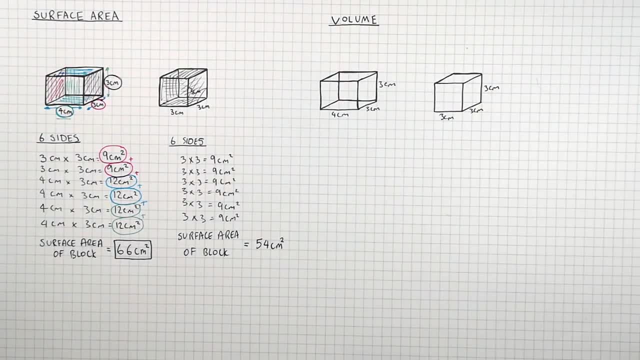 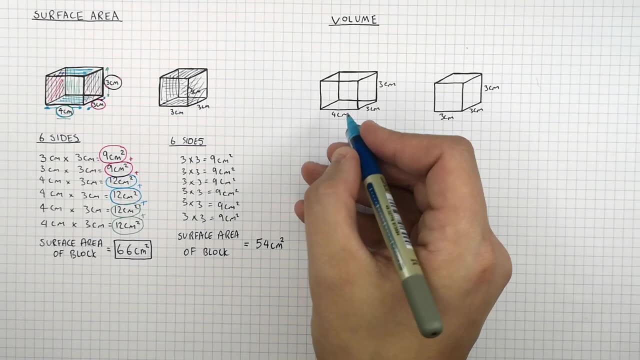 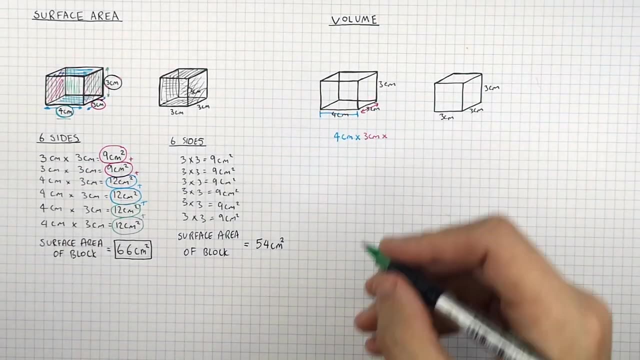 Let's now work out the volume of the cuboid and the cube. To work out the volume, all you've got to do is multiply the length of the cube Length by the width times the height, Which means for this cuboid, you simply multiply 4 centimetres by 3 centimetres by 3 centimetres. 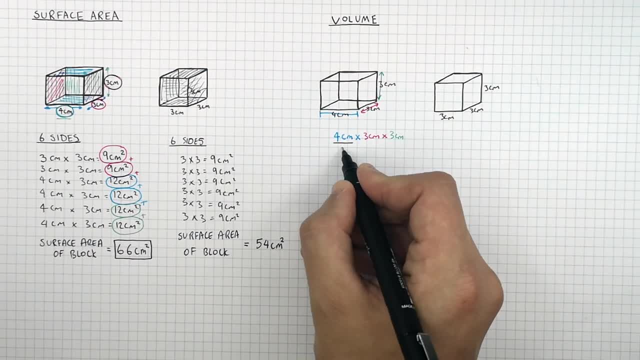 That gives you the volume, Where by 4 centimetres is the length, which you multiply by 3 centimetres, which is the width, which you then multiply by 3 centimetres, which is the height. So the volume equals length times width, times height. 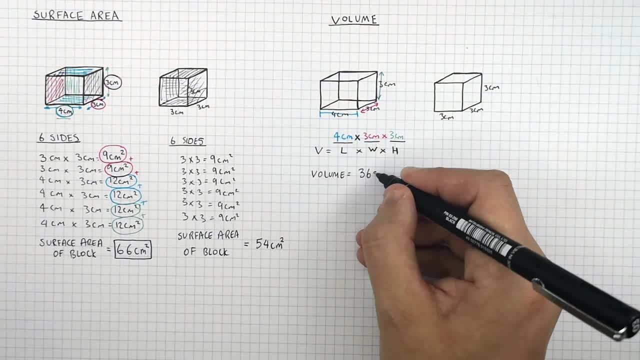 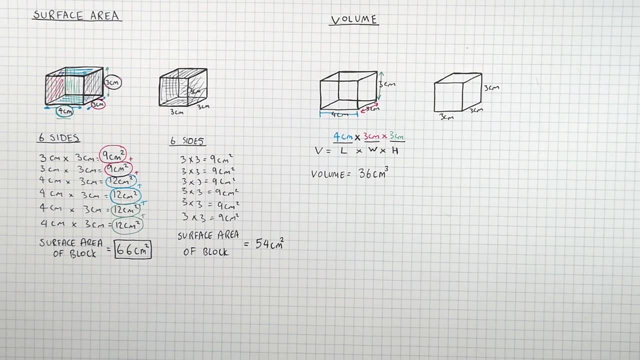 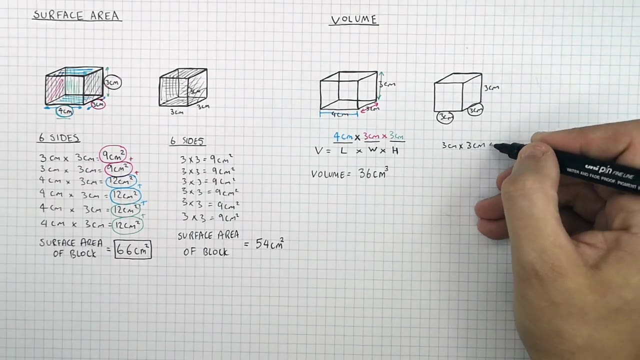 So the volume of this cuboid is 36.. You can see that it's already 36 centimetres cubed. Pause the video to calculate the volume of this cube, The answer will follow. So to calculate the volume of this cube, you simply do 3 centimetres the length times 3 centimetres the width times 3 centimetres the height. 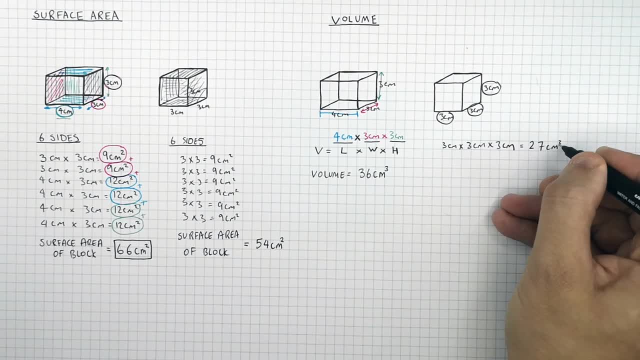 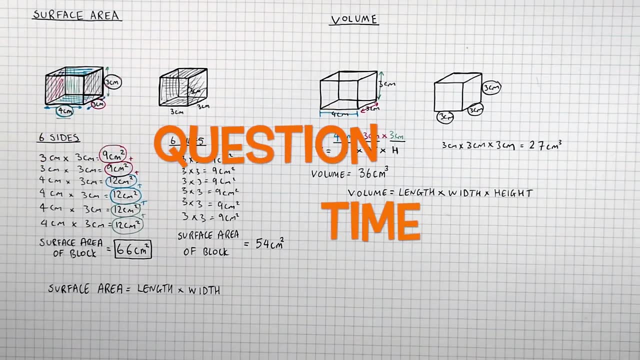 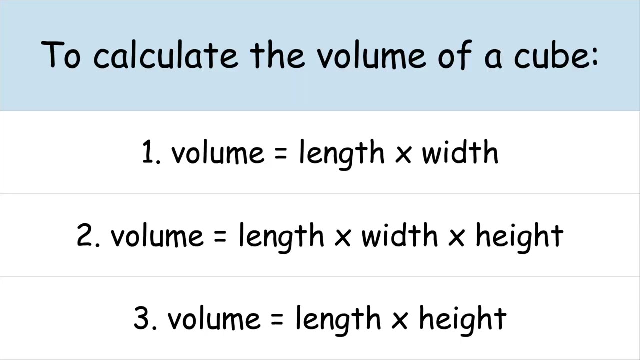 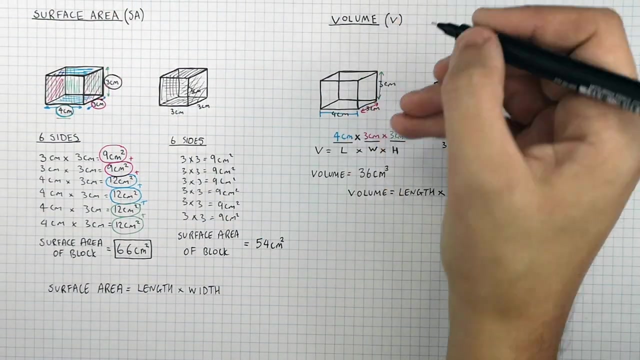 That gives you a volume for this cube of 27 centimetres cubed. To calculate the volume: volume equals length times width times height. It's question time. Tempt these questions to check your understanding. So how do you calculate the surface area to volume ratio? 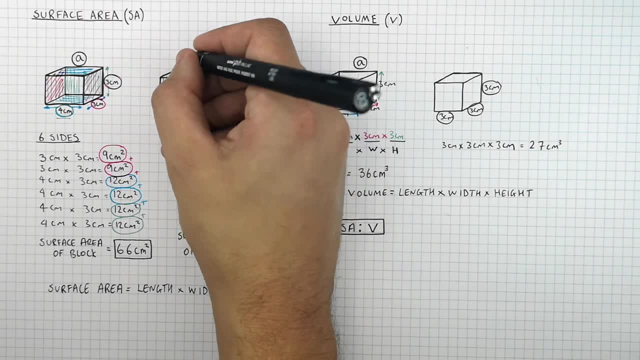 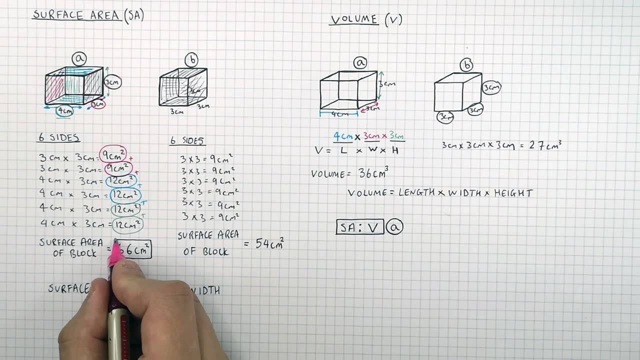 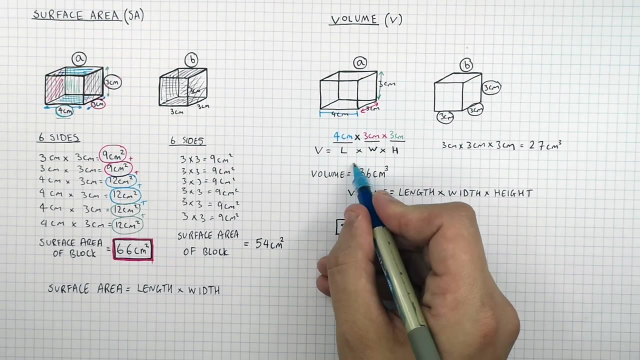 So surface area to volume ratio is simply the ratio between the surface area of an object and its volume. So surface area to volume ratio for block A is going to be the surface area, which is 66cm2, which is 66cm2 to a ratio of its volume which is 36cm3, 36cm3.. 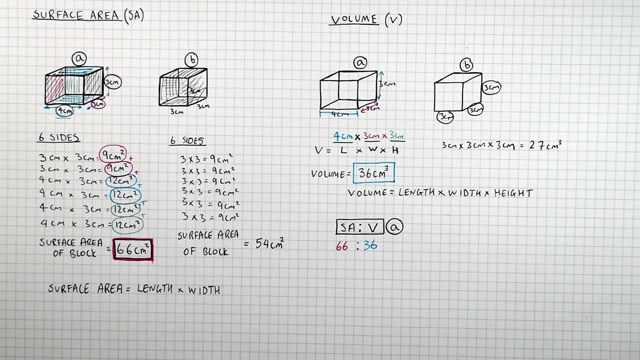 So the surface area to volume ratio for cuboid A is 66 to 36, but we want it as a ratio to 1. So to simplify the ratio, you divide both sides by the volume. So to simplify the surface area, you divide 66 by the volume. 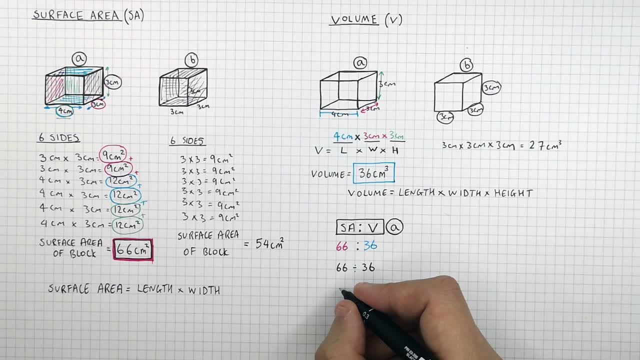 And then, obviously, if you divide 36 by 36, that will give you 1.. Which means that the surface area to volume ratio of cuboid A is 1.8 to 1.. So to work out the surface area to volume ratio of cube B, you firstly write down the 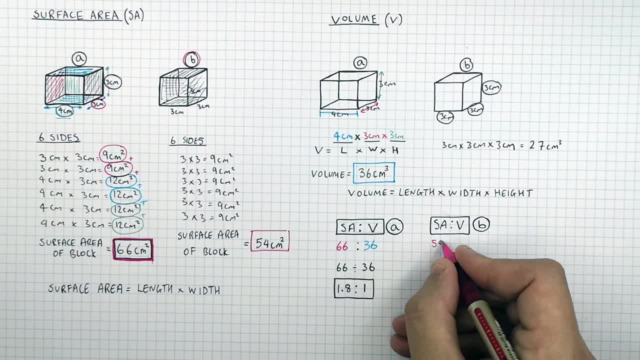 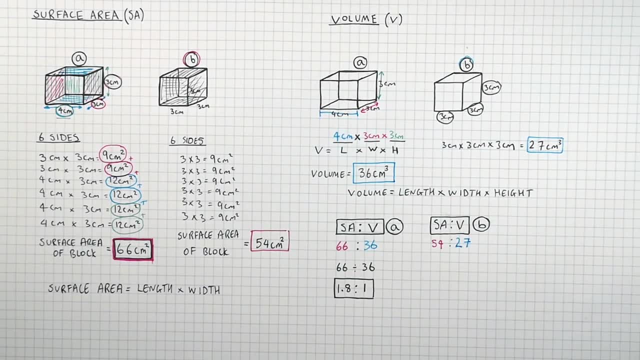 surface area, which is 54cm2.. And then you write down the volume, which is 27cm3.. So surface area to volume ratio is 54cm3.. And then you write down the volume, which is 27cm3.. However, we want to simplify the ratio. 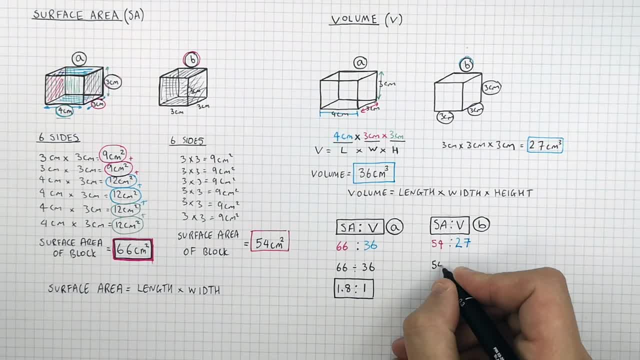 So you divide the surface area by the volume, because 54 divided by 27 is 2.. If you divide the volume by itself, which is 27 divided by 27,, that will give you an answer of 1.. So the simplified ratio for 54 to 27 is 2 to 1.. 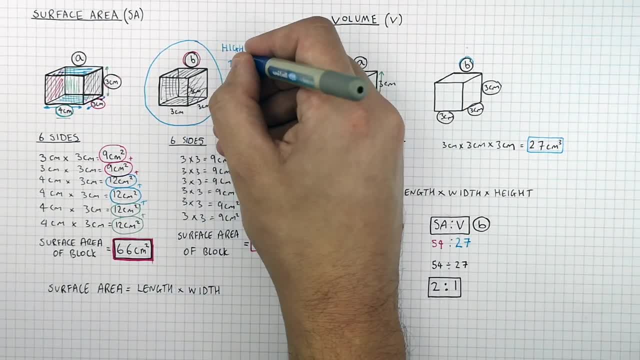 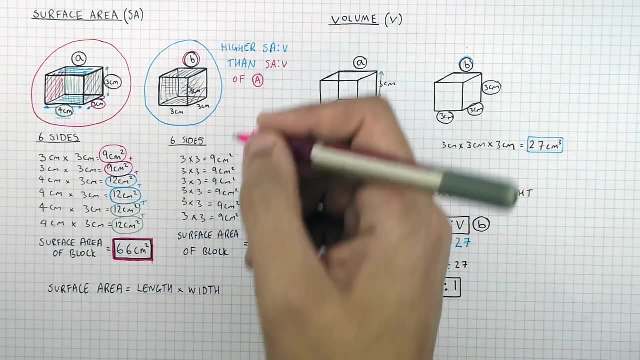 So cube B has a higher surface area to volume ratio, which is at 2 to 1, than the larger cuboid, which is a smaller surface area to volume ratio. So you divide the surface area by the volume, which is 1.8 to 1..